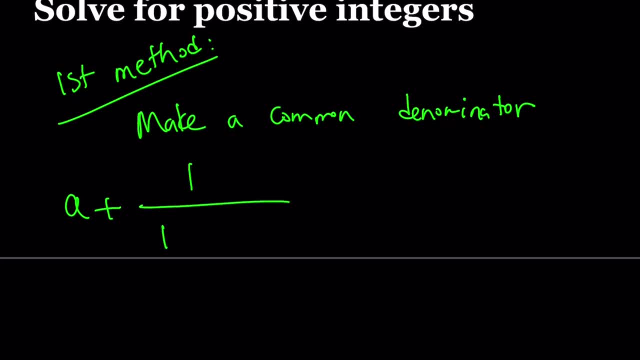 denominator. So start off with a plus 1 over b, plus 1 over c, plus 1 over d, and start at the bottom, make a common denominator and turn this into a plus 1 over b plus and, if you do, a common. 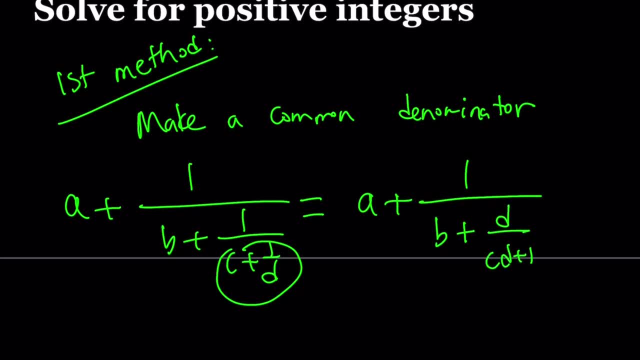 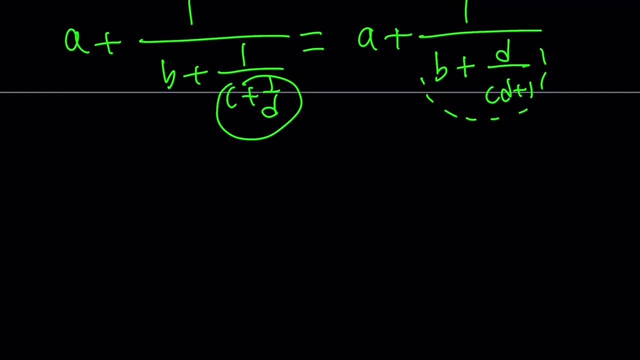 denominator and flip it, you're going to get this expression a plus 1 over b plus d, over c, d plus 1.. And then if you make a common denominator here again and simplify it by, you know, flipping, you get a plus c, d plus 1 over b, c, d plus b plus d, Because what you're supposed to do is b, c, d plus. 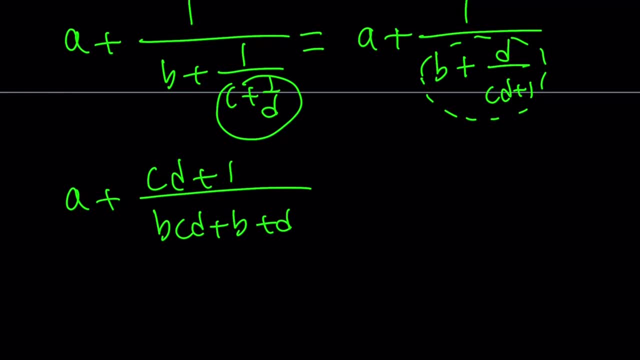 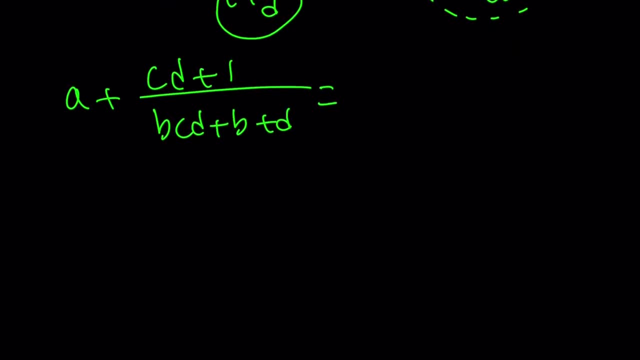 b plus d over c, d plus 1, but then 1 over is just going to give you the reciprocal. That's why I have to flip it. Do it one more time. Do it one more time and you're going to get the following: 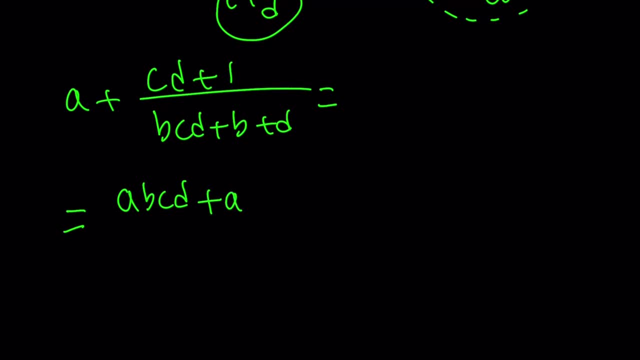 a b, c, d plus a b. Oh, by the way, we have a plus this, so I make a common denominator. There's no more flipping right, We're just going to make a common denominator here. So this part is easy: a: d plus c, d plus 1. 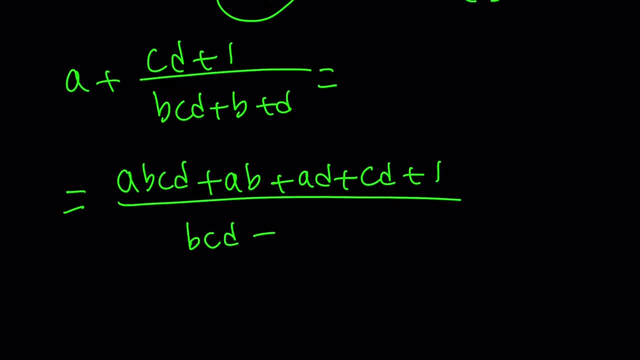 all over: b, c, d plus b plus d. Okay, I was able to make a common denominator completely, and this is equal to 13 over 5.. So a, b, c, there are positive integers. I have a single equation. 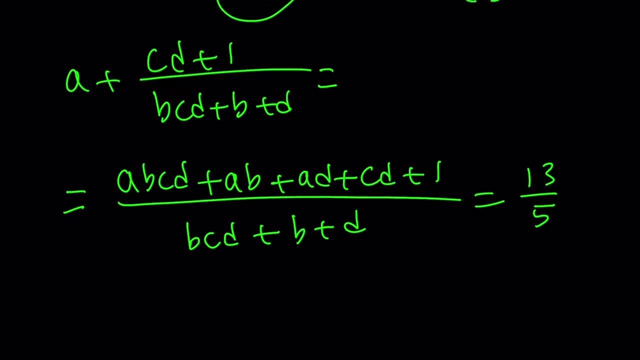 You can kind of think about it as two equations, maybe, like set is equal to 13,, set is equal to 5, but there's also the possibility that they're just multiples of 13 and 5, not just a single equation. So I'm going to make a common denominator here. 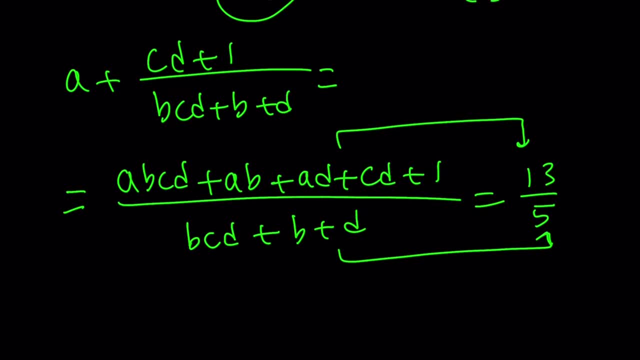 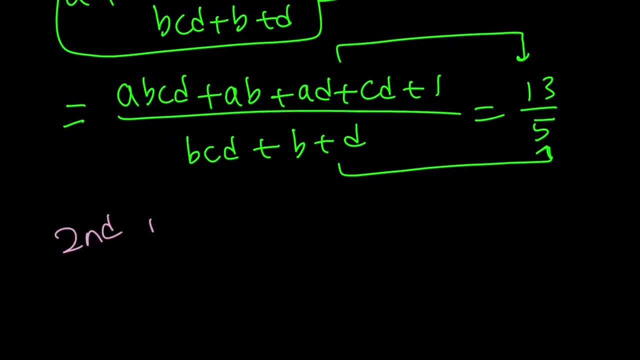 Not necessarily 13 and 5 themselves. right And good luck solving this equation. I'm not going to solve it. There is probably a way to solve it. Maybe this one is a little easier than that. but anyways, as you can see here, this is very painful. So our second method will be completely. 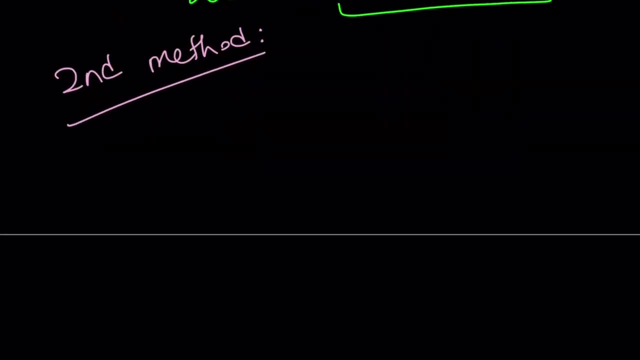 solved, by the way, is going to involve the following. Let me rewrite the original problem: a plus 1 over b, plus 1 over c plus 1 over d. It stops at d, or it can go go on forever sometimes, right? Okay, So to solve this problem. we're actually not going to mess with. 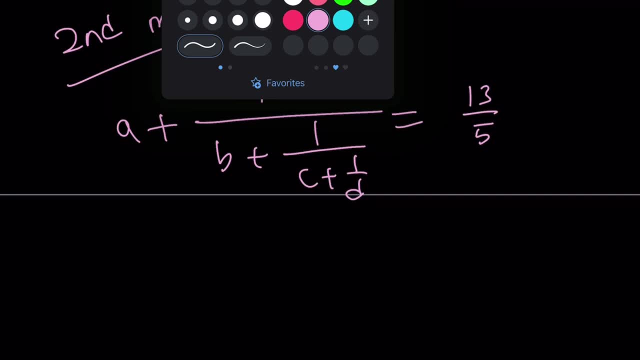 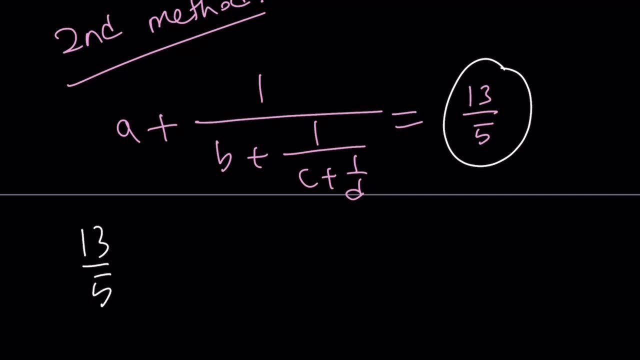 the left-hand side, because that's already very messy and we're going to mess with the right-hand side. So let's go ahead and take 13 over 5 and kind of break it down. So I want to write it as something plus 1 over something, at least right, I mean, I can hopefully like, hey, maybe I can do. 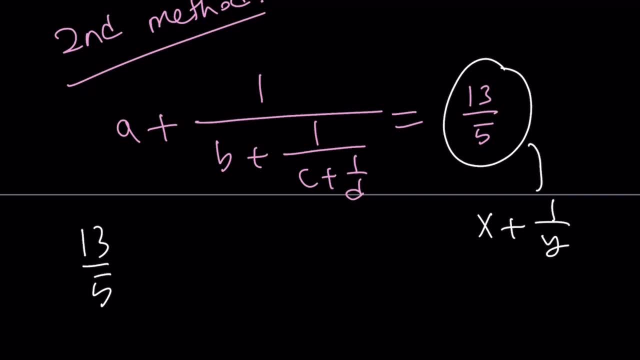 it like x plus 1 over y. Can I do that And then kind of manipulate y but x is a, so on and so forth. So here's what I'm going to do. I'm going to write it as something plus 1 over something. 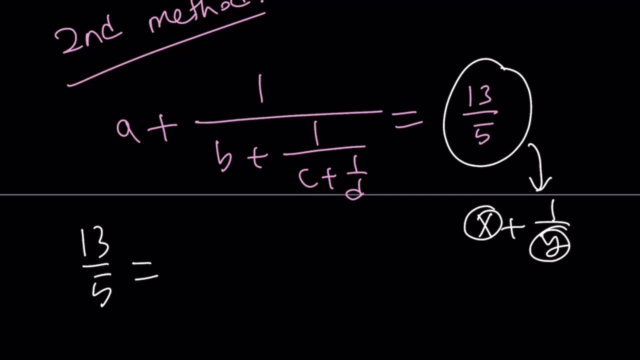 but I'm going to do. 13 over 5 can be broken down into an integer like mixed numbers. I think they're what they're called right. This is equal to 2 plus 3 over 5,, isn't it? Because it's 10 plus. 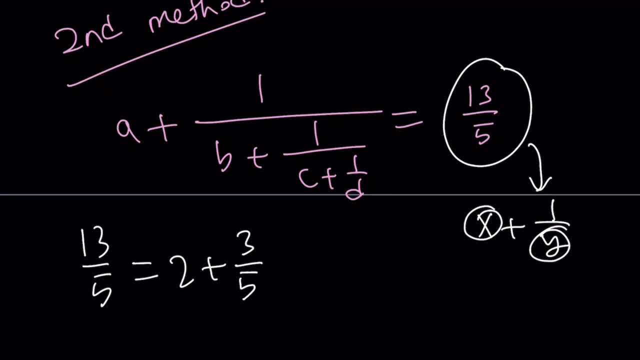 3 is 13,. right. And then here's the trick. We have a 1 in the numerator, so we're going to use the reciprocal of 3 fifths, which is 5 thirds. So we're going to write it like this: 3 fifths is the same. 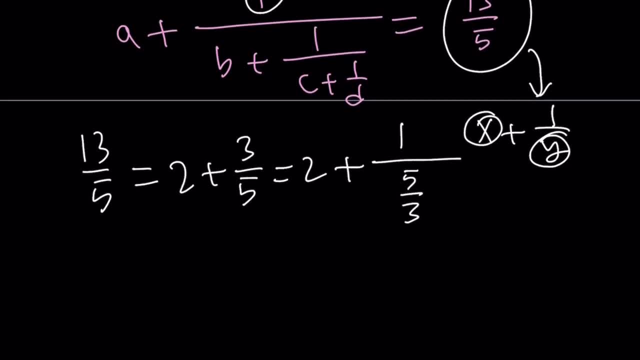 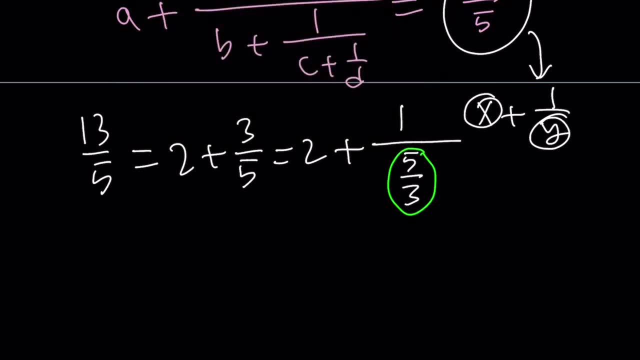 as 1 over 5 thirds, right, And then we're going to take 5 thirds and break it down. We're just going to keep doing it until we get what we want. So 2 plus 1 over 5 thirds can be written as 2 plus 1 over. now, 5 thirds is 1 plus 2 thirds, right, And then we're 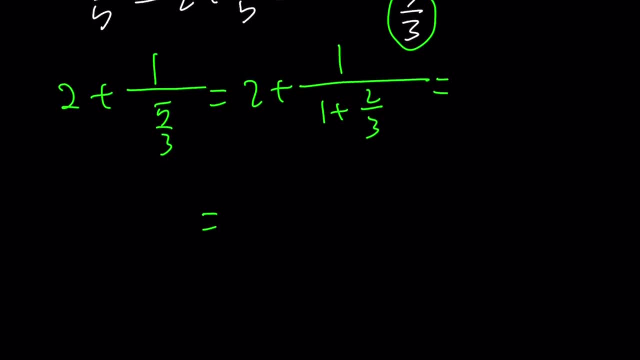 going to write this, as I don't think I'm going to write it there. We're going to write this as 2 plus 1 over 1 plus 1 over 3 halves, So I'm going to manipulate the 2 thirds this time. 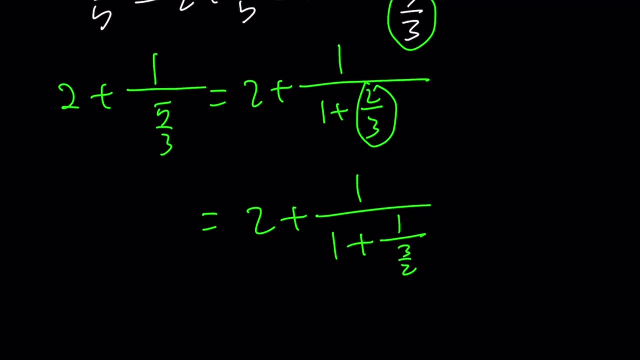 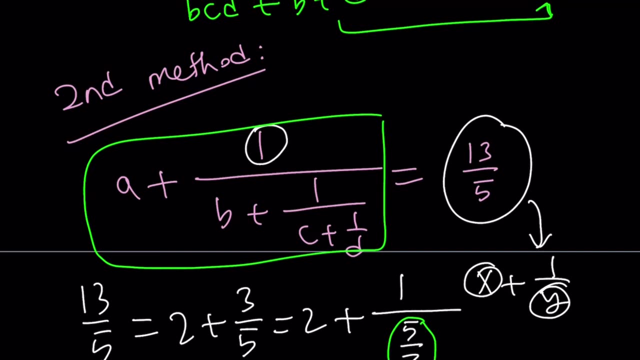 and write it as 1 over 3 halves. The point of doing that is, I want my expression to look like this: right, With that many fraction bars, I have 1,, 2, and 3 fraction bars, And I have 1 and 2 here, so I do need 1 more, So let's go. 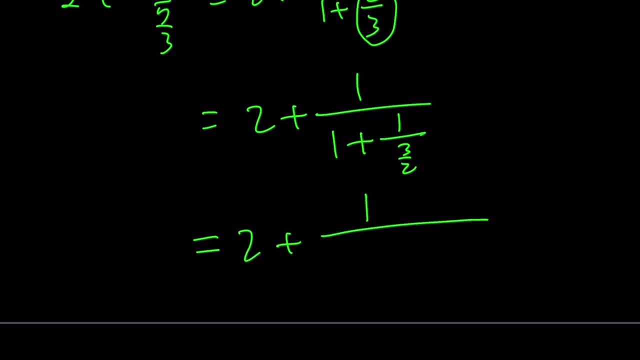 ahead and manipulate this a little bit more. But guess what? 3 halves can be written as 1 plus 1 half and I got 1,, 2, 3 fraction bars and I got the something plus 1 over something 1 plus 1. 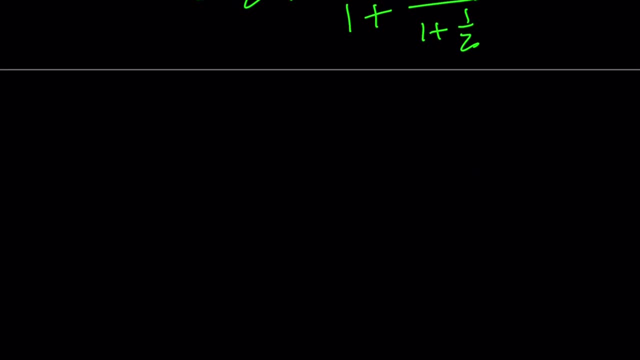 over something, so 1 is over. So I got the same structure. Great, So let's go ahead and write our original equation. The left-hand side gave us A plus 1 over B, plus 1 over C, plus 1 over D. So remember: A, B, C, D are all positive integers. So if you try to,